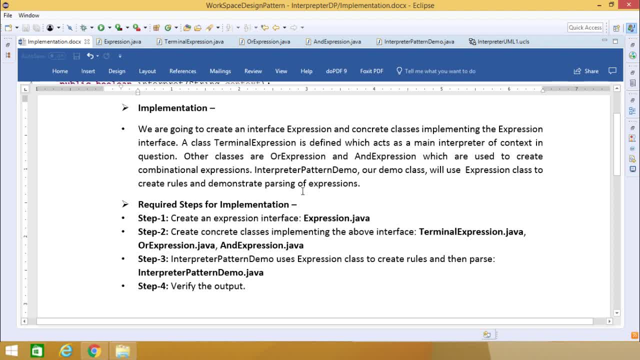 of context in the question And other classes like your or expression and an expression which are used to create combinational expressions. Interpreter pattern demo is our demo class. we will use expression class to create rules and demonstrate parsing of the expressions. So to have a better understanding, let us go through the implementation step by step. 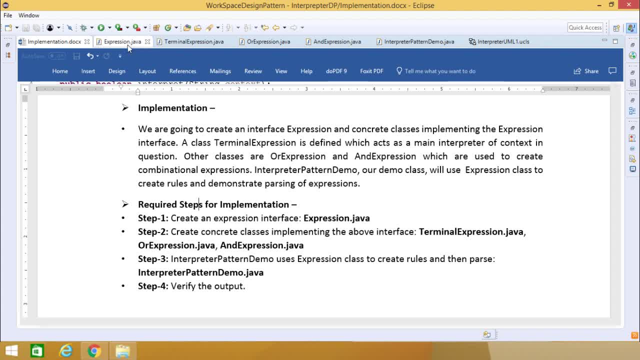 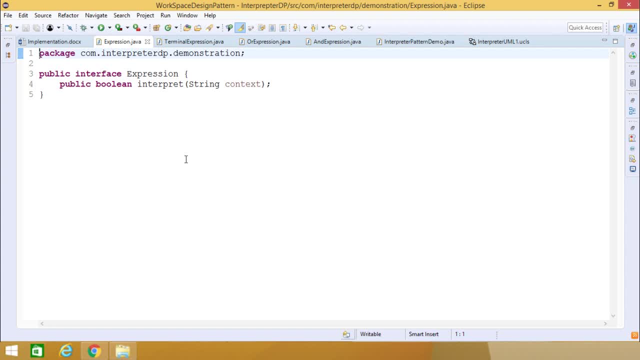 Step number one: create an expression interface: expressionjava. So just see, this is our expression, is an interface which is having one unimplemented method, that is, interpret, which takes string as input parameter and returns the Boolean as output. So now we are going for the. 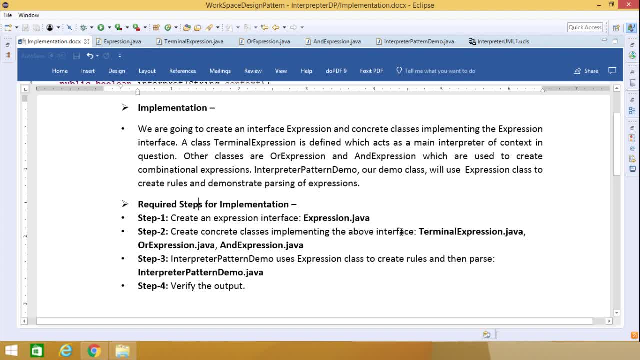 step number two: create concrete classes implementing the expression. So let us go to the next and consider, say, the above interface. So we are having three classes for the implementation of the expression interface. so one is the terminal, expressionjava or expressionjava. 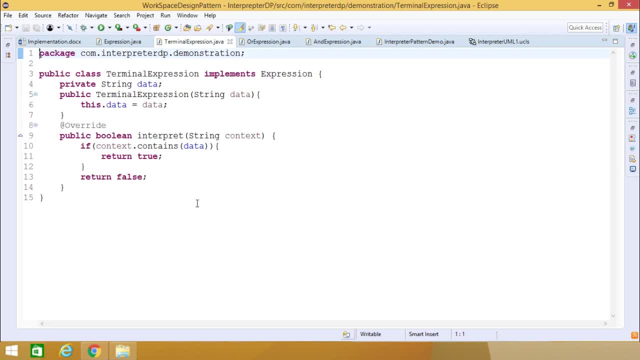 and last one is the and expressionjava. So this is our terminal expression, which implements expression, So it takes the data as input, one instance variable so, of the typed string, this data, and which will be holding the respective data, whatever will be passed as. 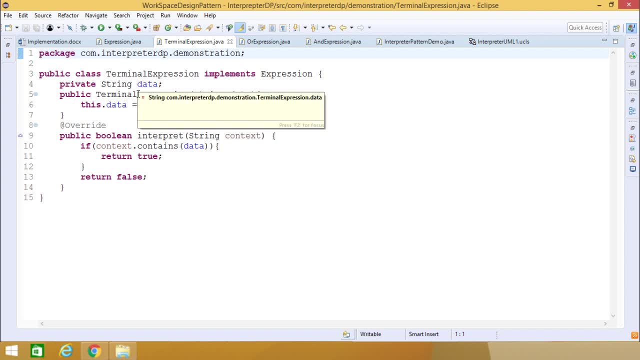 in the parameter as constructor, so that will initialize this member variable. so there is the. this dot data is equal to data and also we have implemented the interpret function which was there in expression interface. so this is the respective code. so one string will be put as input argument. so context dot contains data. so if this particular context string object. 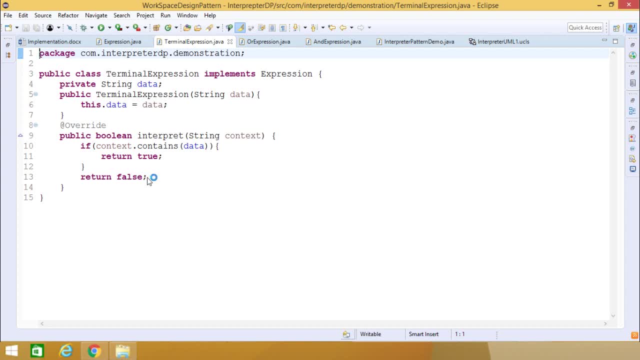 contains this data, then it returns true, else it will return false. next we are going for the or expression. so here we have defined two expression objects: expression one and expression two: expr one and expr two. this is the or expression constructor which will initialize this: expr one and expr two. this is a interpret. the method has got implemented here, so we are going for: 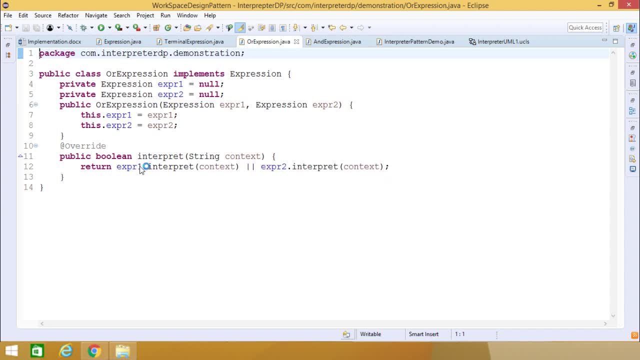 the whatever the string which will be passed. so expr one dot interpret context and expr two dot interpret context. so in this way the respective string will be passed. so here, expr one and expr two. they are nothing but the expression objects and they have got initialized through this parameter. 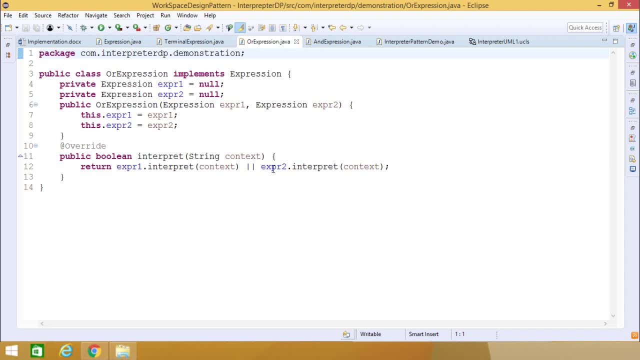 as constructor. interpret is a function which has got overwritten like this. similarly, we are going for this and expression. so before going, just remember: in case of or expression, we have used this logical or operator in between. so now, in case of and we have done the same only. 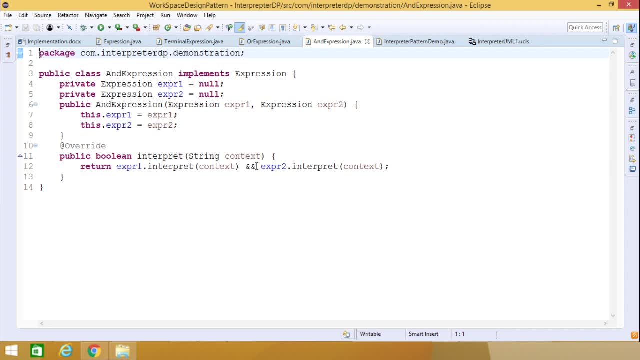 here this: we are having this logical operator ampersand. ampersand that is denoting the and. so one string input argument. and expr one dot interpret context. and and expr one dot interpret context. so we have- we have discussed this expression interface- one concrete class that. 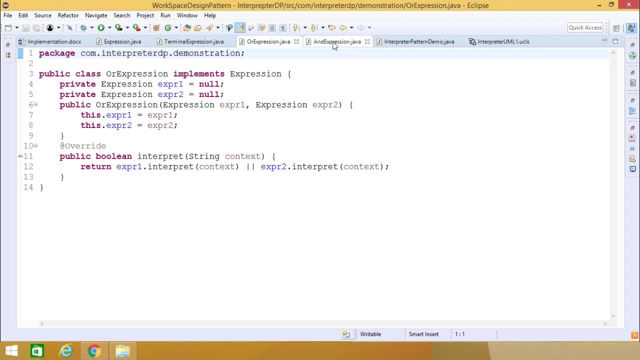 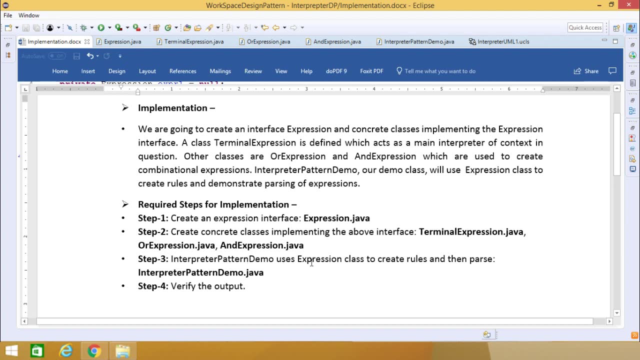 is a terminal expression, another one is the or expression and the last one is the and expression. so now we are going for the step number three. interpreter pattern. demo uses expression class to create rules and then parse, and that is our interpreted pattern demo dot java. so that is the class here we are having. so this is the 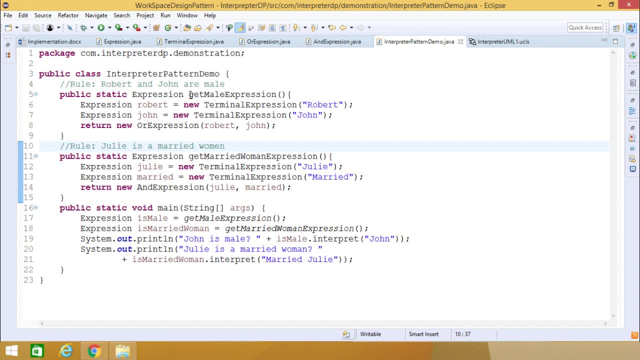 interpreter pattern demo. so it is having one method, that is a get mel expression. so here we are having this new terminal. expression is an input argument is robot is instantiating this expression, object robot. and here we are having this expression: john, here is equal to new terminal. 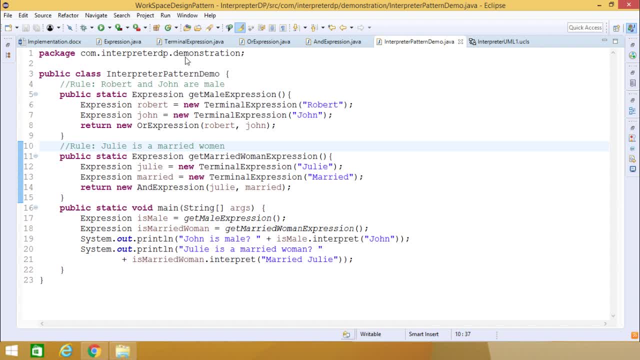 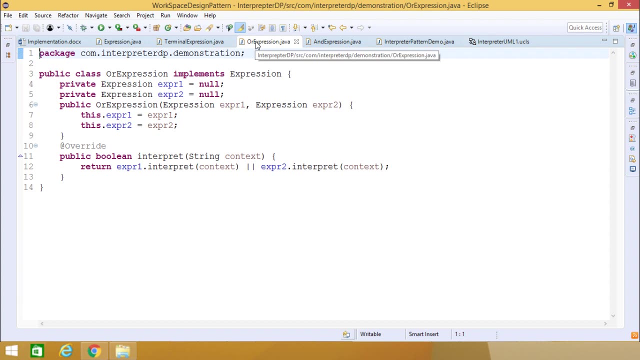 expression john. so here we are passing this robot and john. so obviously they are getting assigned to the respective data. now return new or expression: robot comma, john. so we are passing these two expressions as input argument for this or expression. so here you can find that this: these two expressions will be assigned to the instance variable expr1 and expr2. 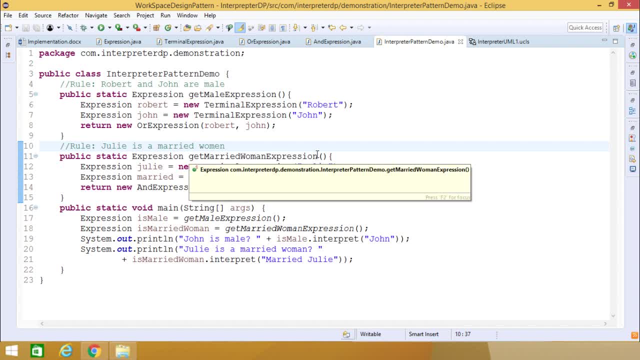 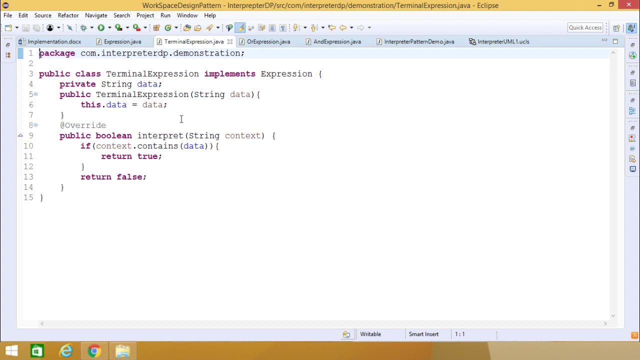 okay, now we are going for this get married woman expression which returns one expression. so expression object julie and expression object married. so here having this terminal expression julie and terminal expression married. so what will happen in case of terminal expression through this constructor, julie and married will get assigned to the data respectively accordingly, and then 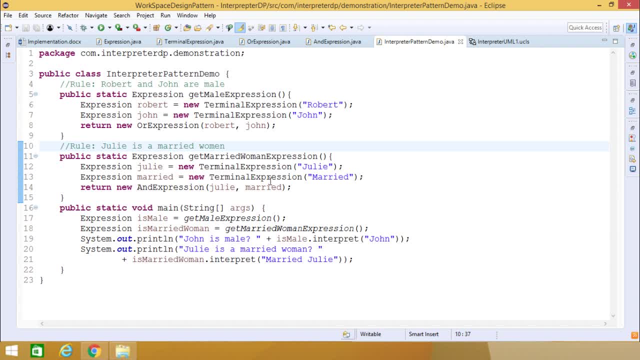 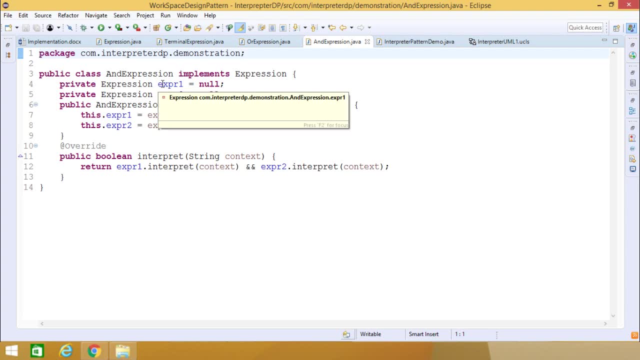 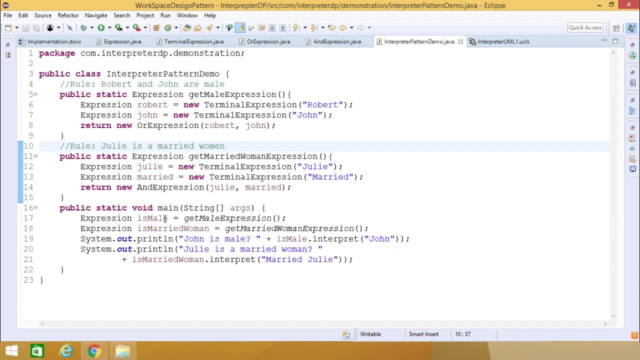 we are calling this and expression, where we are passing this julie and married. that is the expression. class objects as input arguments, so now, so here. so they will be assigned to the respective expr1 and expr2. now we are having this main function, so expression is. 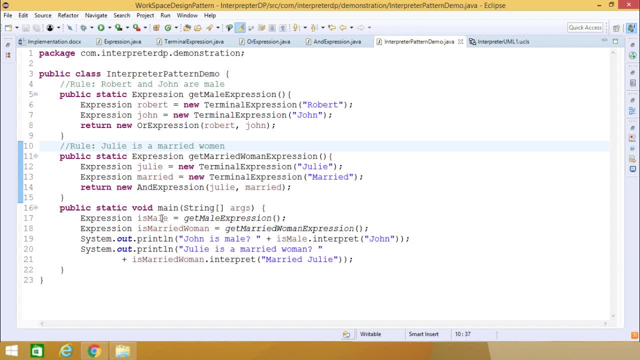 male is equal to get male expression. so is male is holding that output argument of this: get male expression. so that means the all expression output. and then we are having this: is married woman is equal to get married woman expression. so now we are going for systemoutprintln. 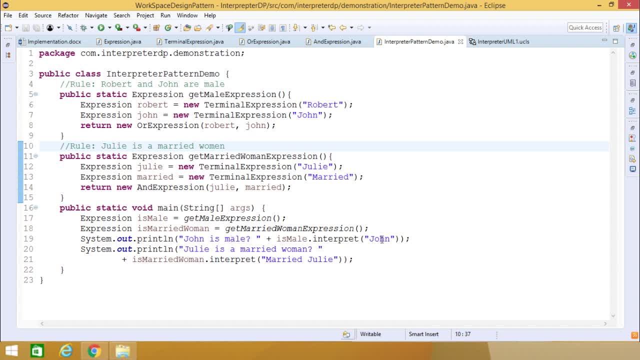 john is male. so here we are passing this john is male dot interpret john. so this male is expression object which has got instantiated by the output argument of this get male expression. so now this john is there, which is which is supposed to get interpreted here. so now what? 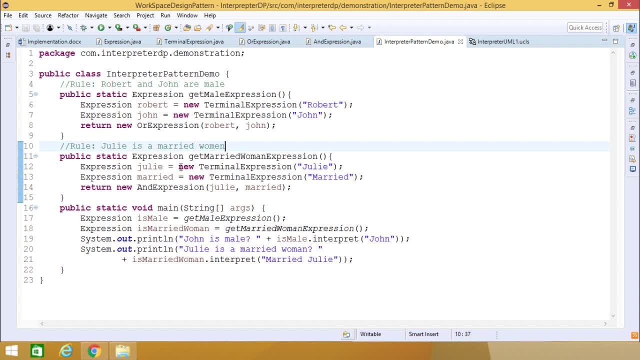 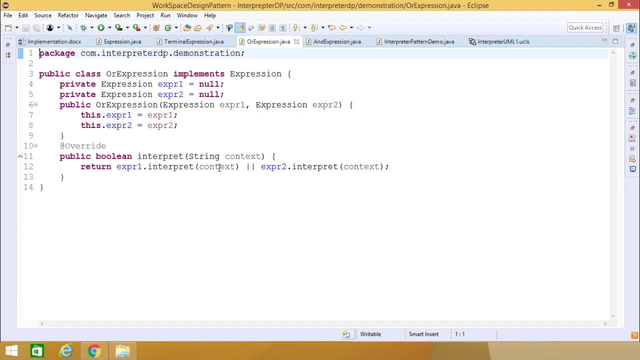 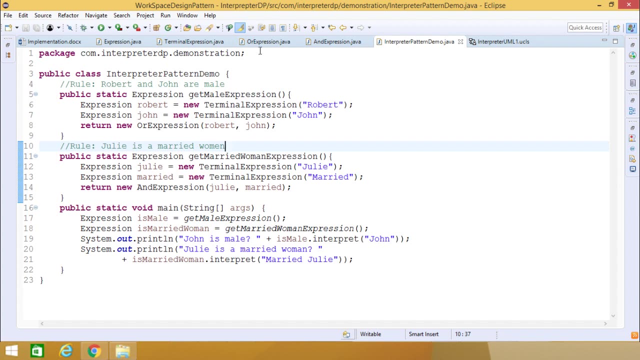 will happen if you go for this. you know the in case of get male expression. we had that or expression there, so we are going for this or expression. so this is the context. we are passing, this interpret we are passing here, so this interpret is containing this: john. as a result, 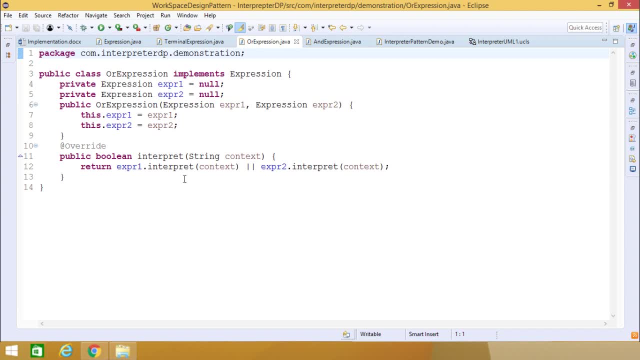 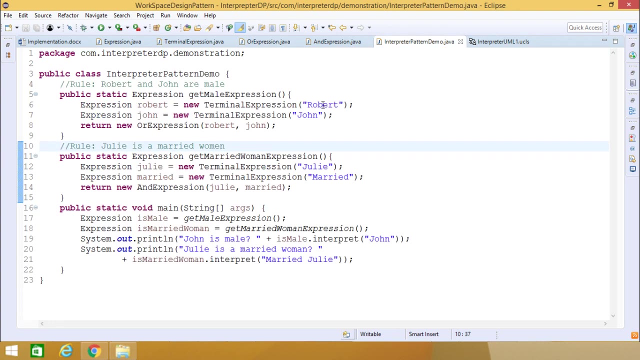 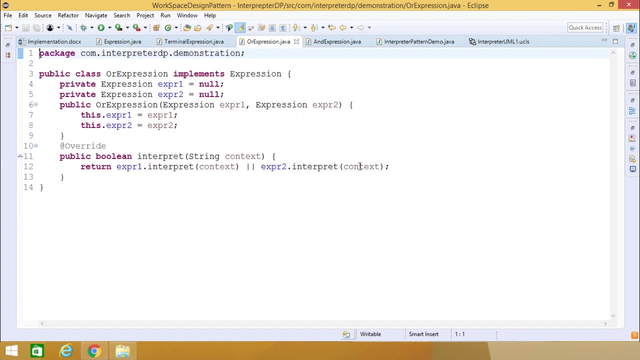 of that, this particular, this particular context, and it will be- will be going for expr1, expr1, dot interpret context or expr2, dot interpret context. initially, expr1 and expr2 in this case was got initialized with the robert and john, so that's why this john will have a match here is john will have a match here. so here we're. 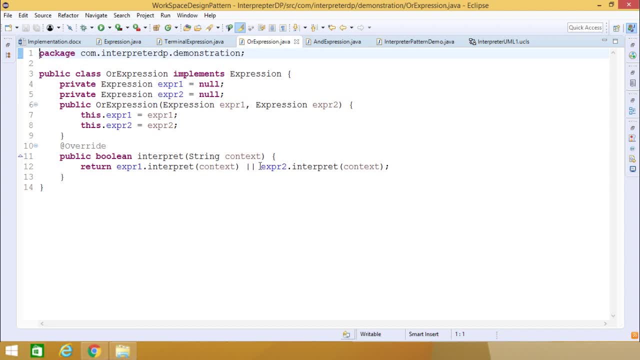 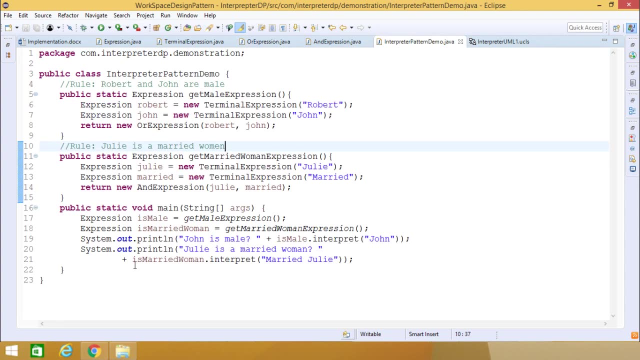 having this robert and john, so john will have the match here. so all logic is there. so one is false, another one is true. so true will be the outcome. true will be the outcome here and similarly we are going for is married woman dot. interpret married julie, so you can. 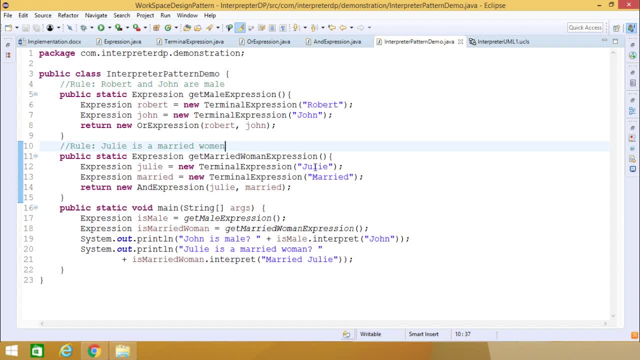 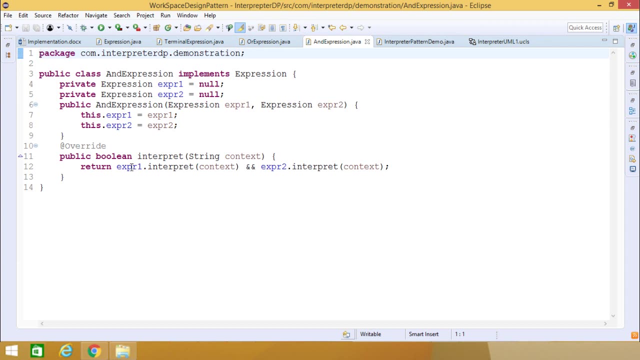 find this married. we have put that one here and this julie is also there. so here we are going for. this interpret is married woman, so i'll be coming to this and expression, because it is the and expression was there. so that's why, in this particular context, we are having both julie and married. so exp1.interpret. 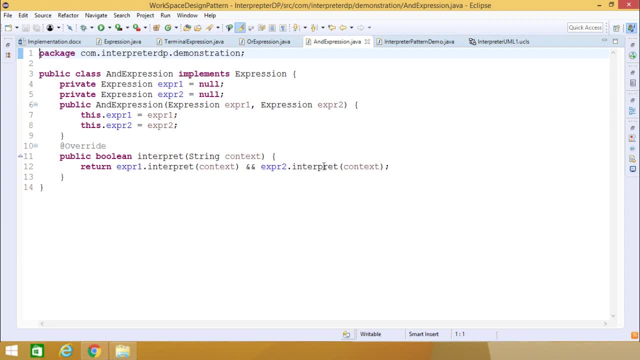 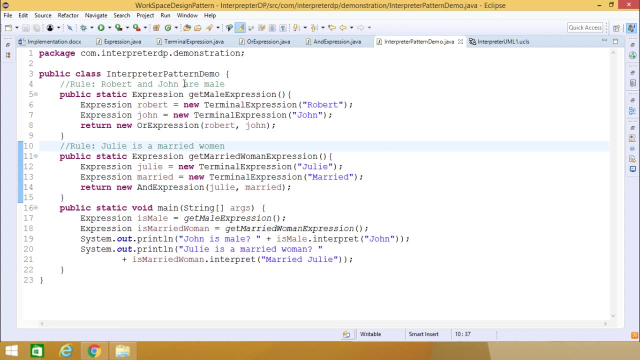 context will return true and exp2.interpret context will be returning true, true and true will be true, so output will be true here. so in this way you are going to get this respective output. so here you can find the outputs are true and true. so in this our implementation, we have